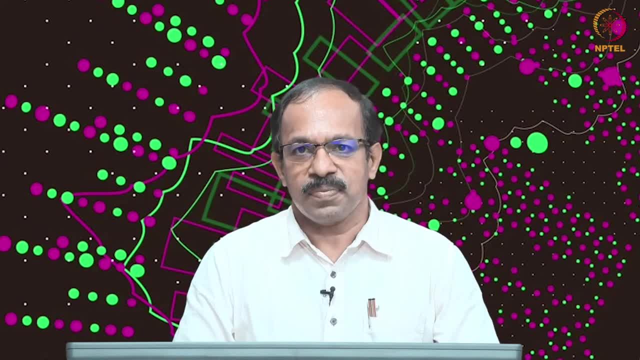 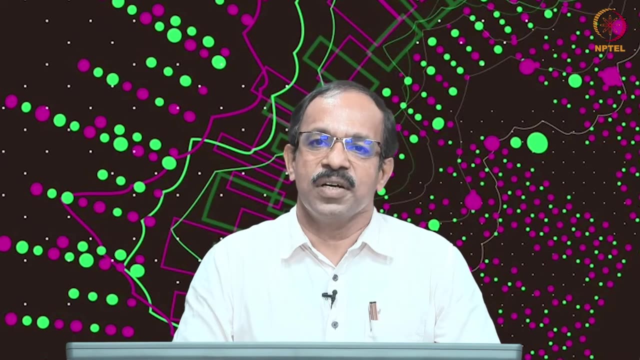 developing autonomous robots also will be covered. In the last few classes we have been listening to the details of mobile robots, the wheeled mobile robots, its construction and the kinematics, And by now you know that mobile robot can actually move around. it can actually do many. 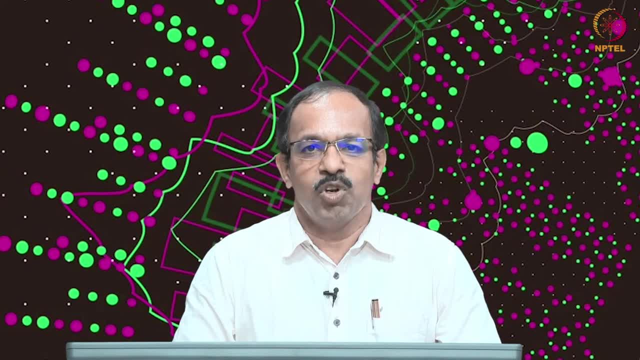 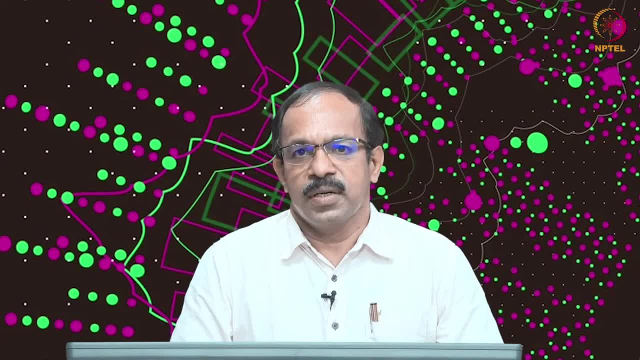 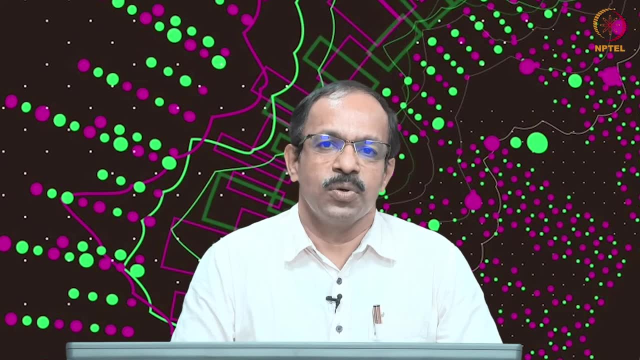 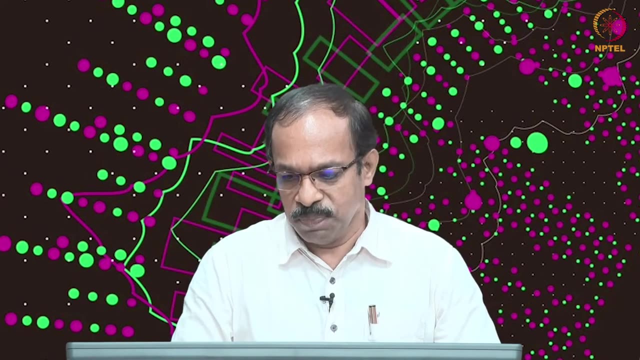 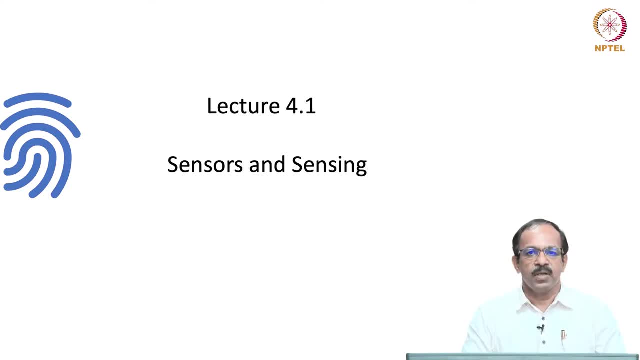 focusing on sensors and sensing. So what are the different types of sensors used and how they actually do the sensing in the environment? that is going to be the focus. But before going into the sensors and sensing, let us look at why do we need sensors in robots? 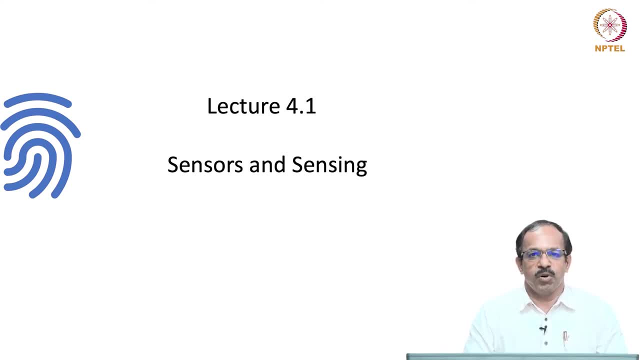 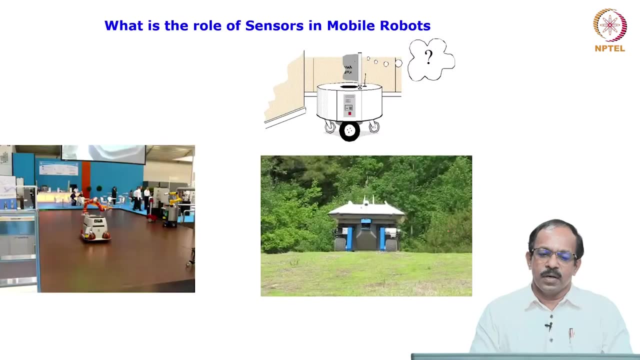 or what is their role in the overall application of mobile robots for various applications. As you know, there are different kinds of mobile robots available and some of them are remotely operated, some of them are autonomous, some of them are omnidirectional. So you will see that robots vary in their construction and their application. 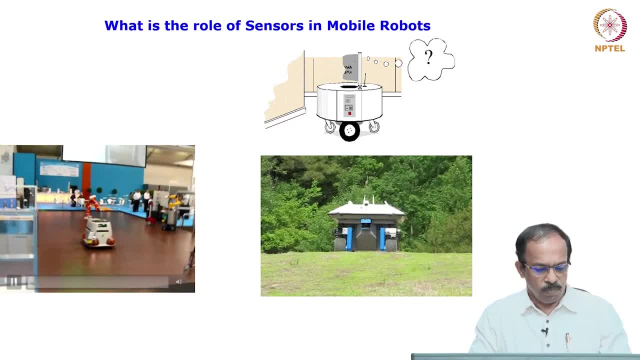 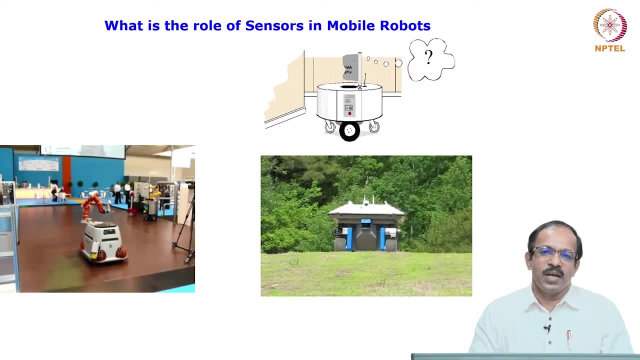 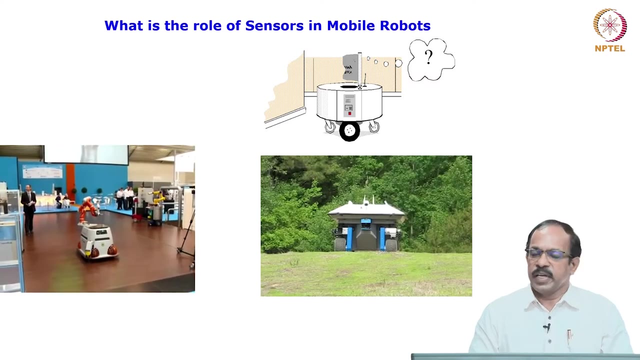 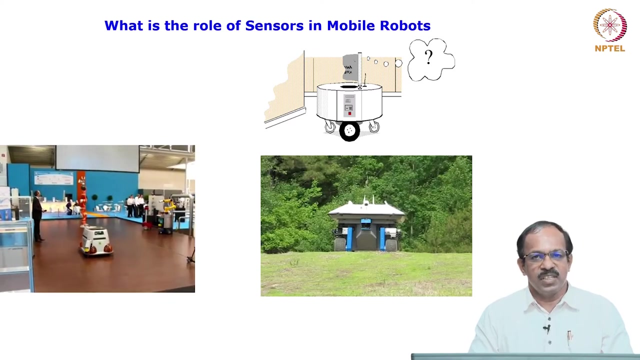 As you can see here in this one, you will see that this is a mobile robot with a manipulator attached to it. Except for the manipulator, it is like a robot. It is like a normal mobile robot And you can see that the robot has to do many tasks in this environment. 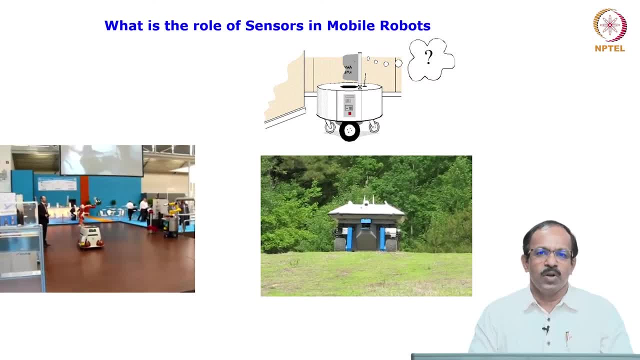 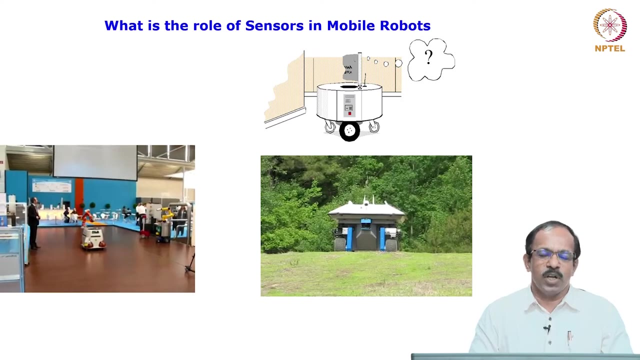 So sometimes the robot has to go and pick up something, sometimes it has to insert something on a workpiece, or sometimes it has to do some inspection of some objects. In all these things the robot has to make many decisions. The robot has to see whether it can actually identify the object. 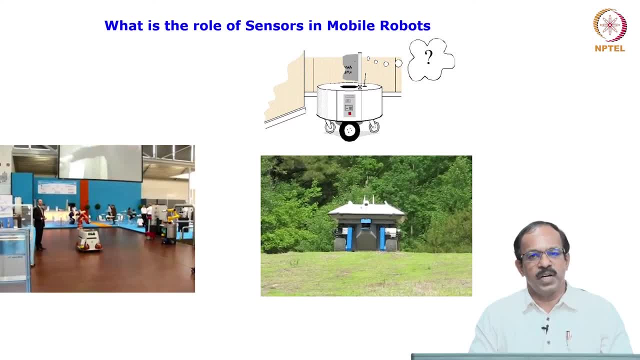 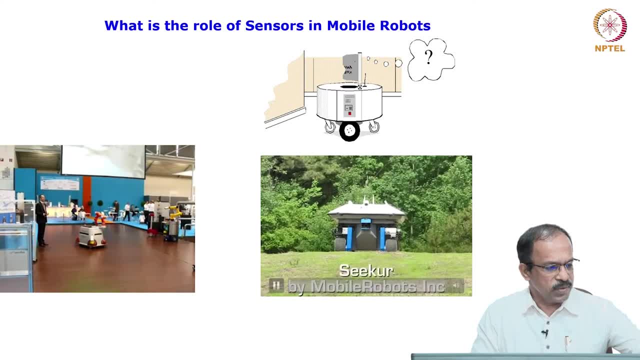 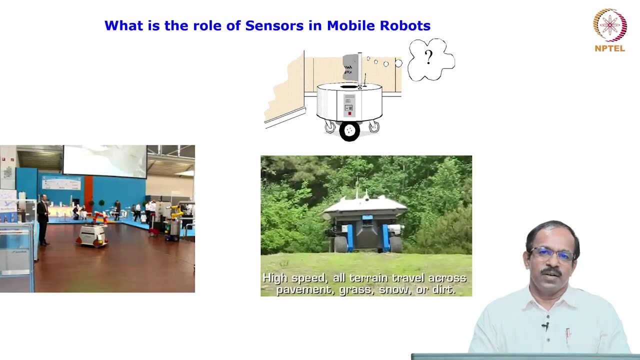 Now you will see that the other robot, what you are seeing here, which is actually a omnidirectional robot- we call this as the- it is a seeker robot. it has got four wheels, and you can see that the four wheels are steerable as well as it is powered also. 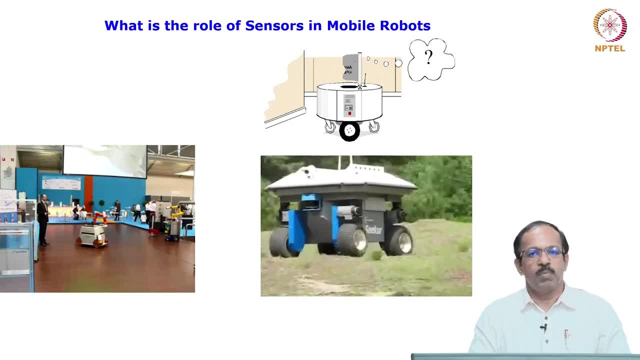 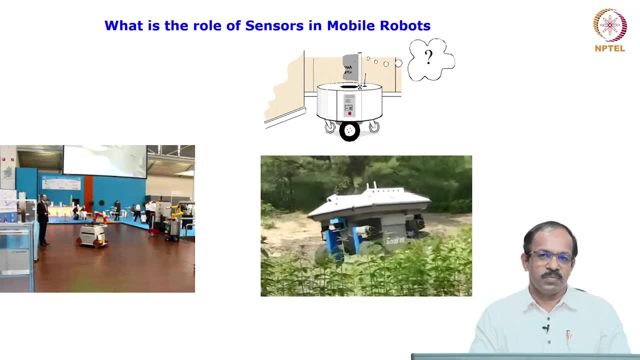 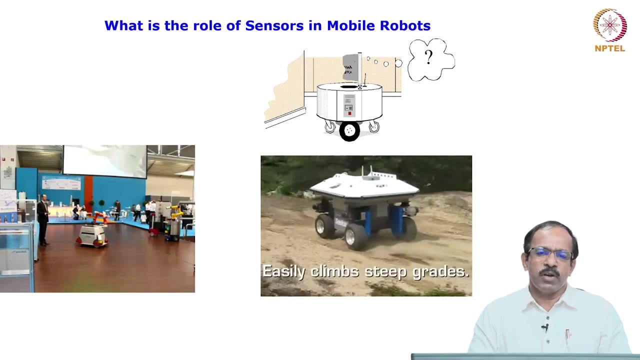 So with this kind of configuration, the robot can actually have omnidirectional motion as well, as it can carry out the tasks which are assigned to it, And you can make it fully autonomous also. So we will see when we talk about the remote operation and autonomous operation there. 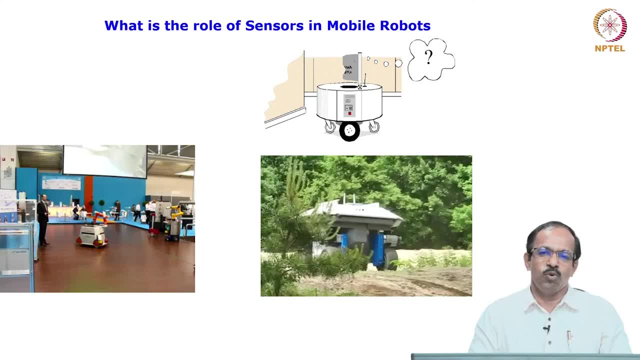 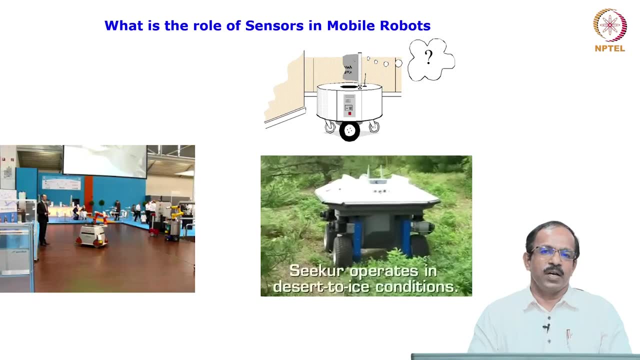 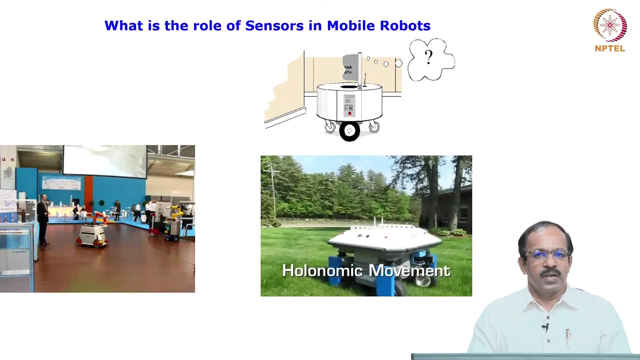 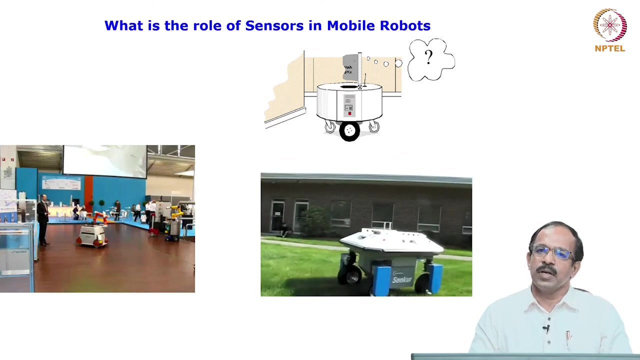 are major differences in the way the robot has to behave In a remote operation. as you know, the robots just need to follow the instructions given by the operator. whether he is sitting close by or far away does not really matter, And there is no need of information processing or decision taking in the case of remotely. 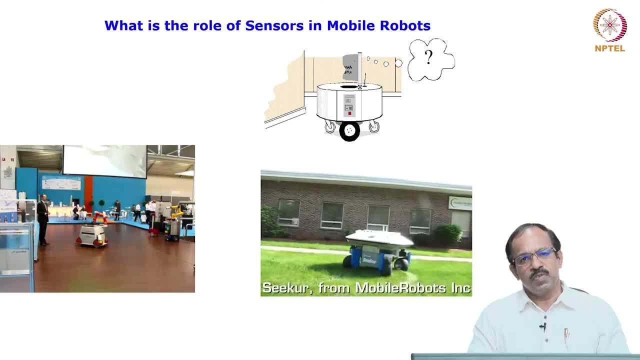 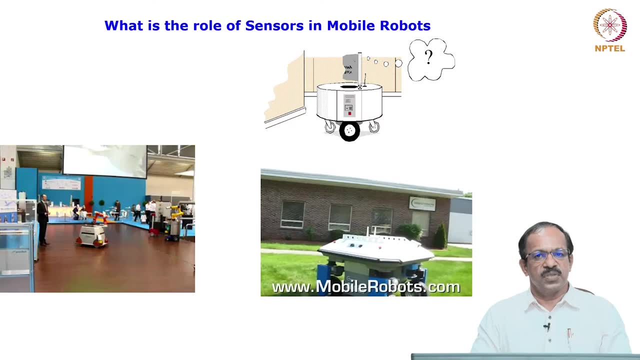 operated robots, But in the case of a mobile robot which is autonomous, there are many other things the robot has to do, And this can be done only with the help of a remote operator. The robot needs to have different kinds of sensors and process the information in order. 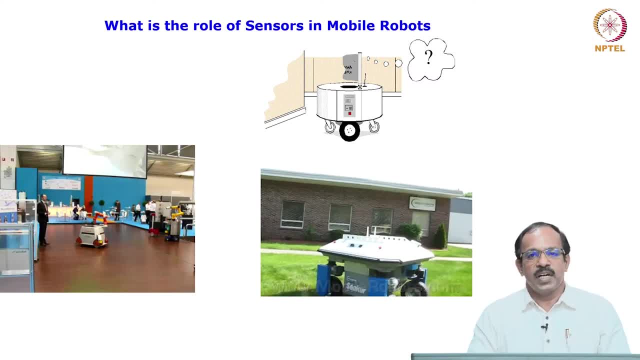 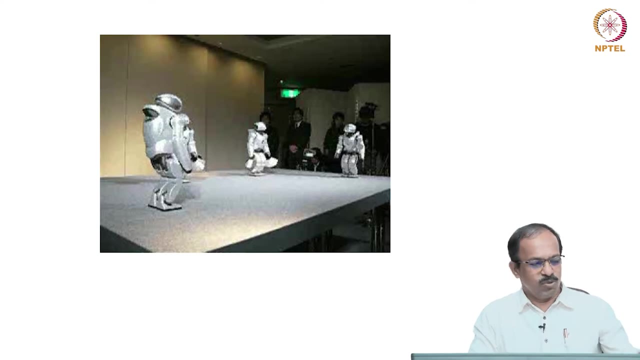 to take a decision or even to know where it is and then to take decision and then execute its decision. So this is one of the important requirements of a mobile robot And for autonomy. we know that there are many things to be understood, For example, as you can see here in this video. so it is not only the robot on its own, but 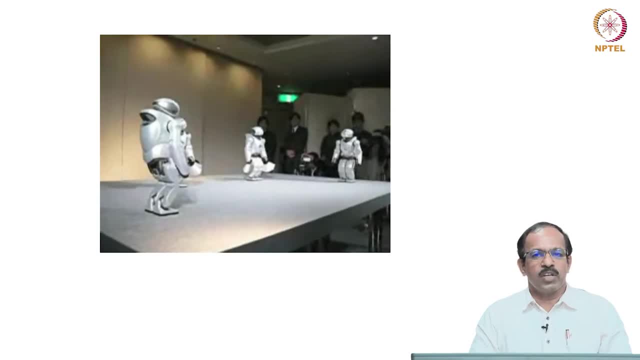 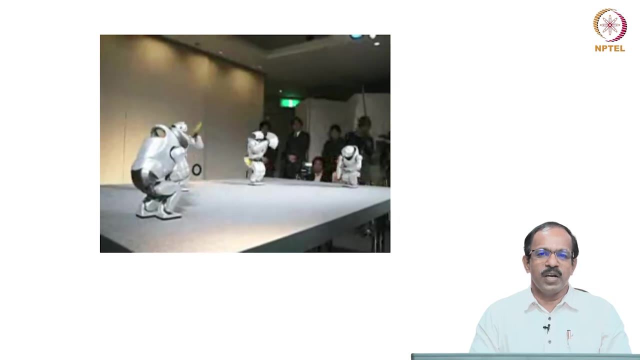 the robot. if it has to be autonomous, you can see that the robot has to collaborate with other robots also, or they need to have coordinated motion also. So if it is fully programmed, the robot has to understand what is the environment, what is its surroundings, how the other robots are behaving and based on the other robots. 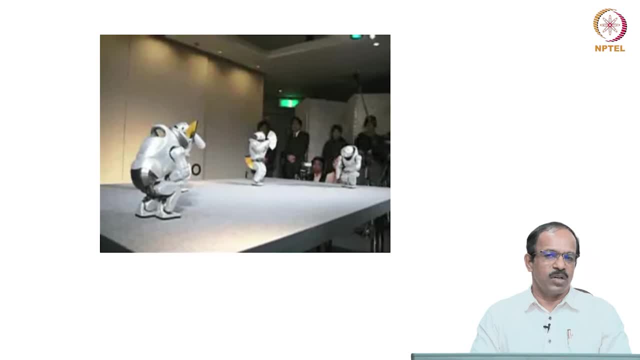 behavior. the robot has to adjust its own behaviors also, So in this case it is fully programmed. Online decision making is not there. In case there is an online decision making needed, then the robot has to observe its surroundings, understand the surroundings and then make decision. 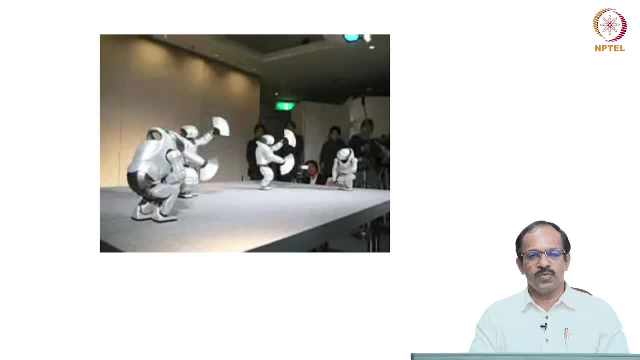 So all this requires sensors. So sensors are one of the major requirement. in a mobile robot- or, for that matter, any robotic system, sensors play a major role, But in the case of mobile robot, it plays an important role because of the perception it needs to have around surroundings. 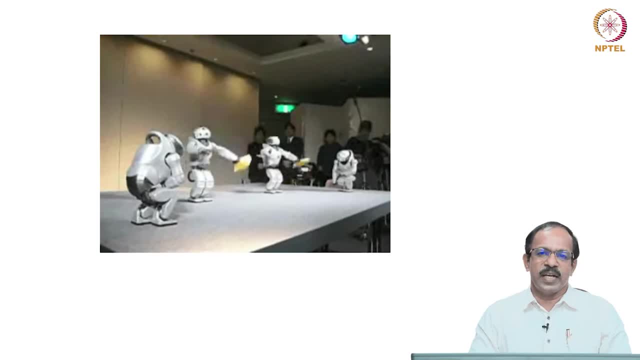 The surroundings are not the same, unlike an industrial robot where, once you fix it, the surroundings will not change drastically, But in the case of mobile robot, there is a large change in the surroundings And that is why we need to have the sensors in order to give a perception of the environment. 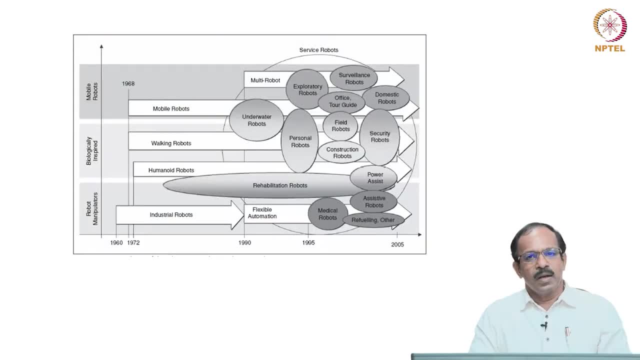 to the mobile robots. So what are these kinds of mobile robots that we are talking about? this is just to tell you about how the robots evolve. Okay, So we are talking about how the robots evolve over a period of time and how that is actually. 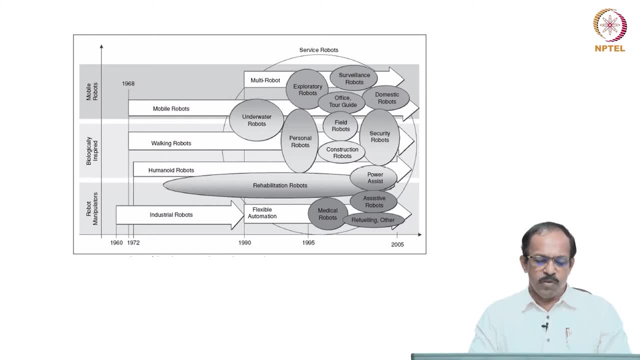 changing the way we look at the sensors and the perception. If you look at the robotics growth or the evolution of robotics, you can see that it was only in the 1960s or 70s we got the industrial robots. Yes, industrial robots also needed sensors. they wanted to have contact sensor or proximity. 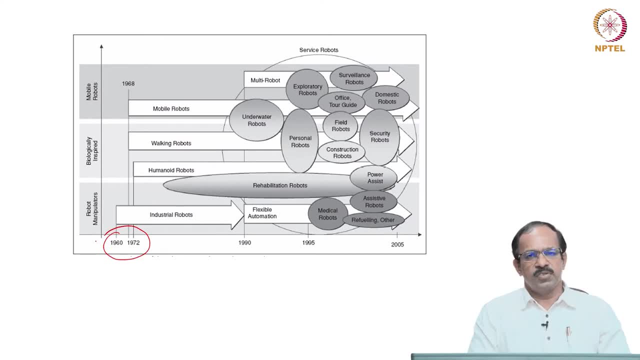 sensors, touch sensors, etc. In even vision sensors, sensors were added to add some attention. So we have the technology to add some additional capabilities. Over a period of time we had a lot of development in the case of industrial robots and a lot. 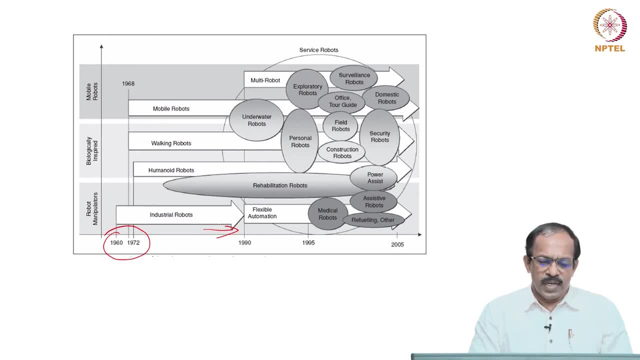 of technologies were developed. Later on, we realized that we are still not able to go to the people or we are not able to go close to the human with the industrial robot, and that is where we got this service robots, or we call this field and service robots. 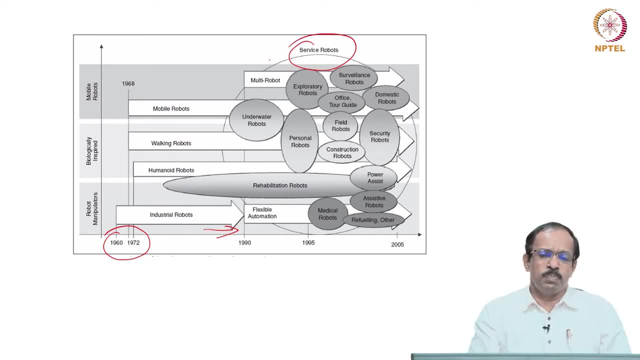 This field and service robots are not the same. They are not the same. They are not the same. So these robots play a major role now because all the technologies, what were developed for industrial robots and the technologies developed in the research centers for mobile robots- 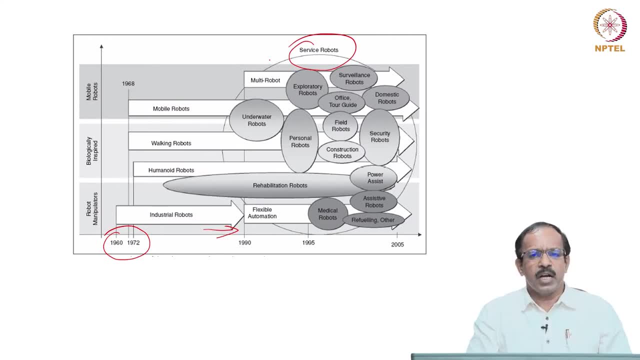 working robots and humanoid robots they have. they come handy in developing new applications for robotic technology, and that is why we have underwater robots, we have security robot, we have field robots, we have surveillance, We have aerial robots, We have medical robots, medical robots, etcetera, etcetera, and all these robots, some of them. 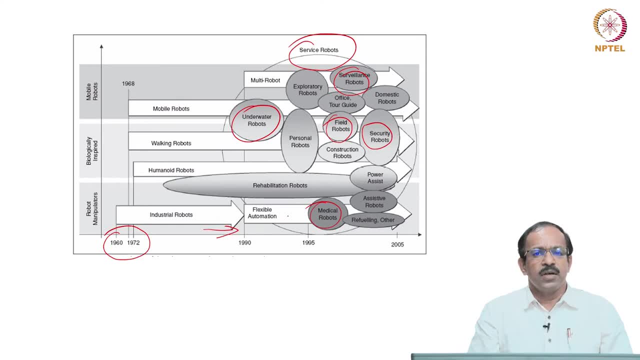 are mobile. some of them are not mobile, but whatever may be the case, we have an important requirement of sensing and perception. Without sensors and without perception of the environment, no mobile robot can actually work, and that is why we need to understand the various kinds of sensors and how these 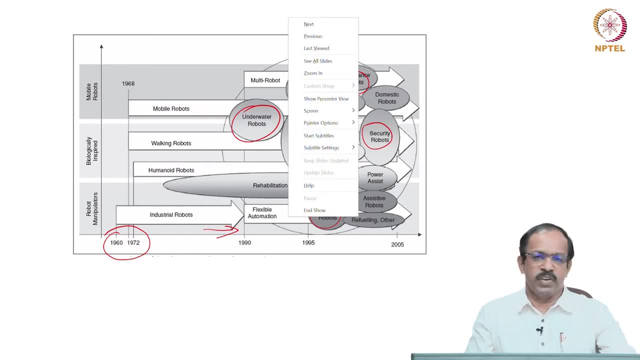 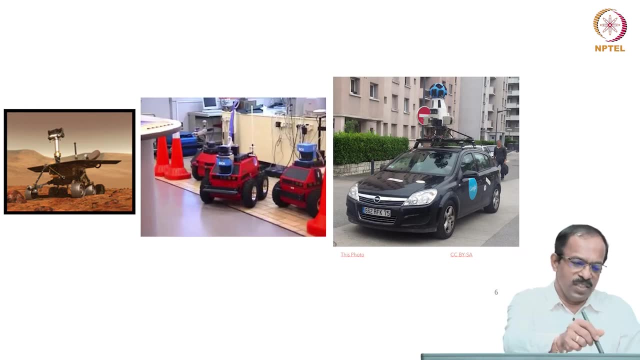 sensors are used for mobile robot navigation. Yes, You can see there are some of these robots here. So, as you can see here, the first one, this one is the rover, the Mars rover, and then you have these autonomous mobile robots, wheeled robots, and most of you know about. 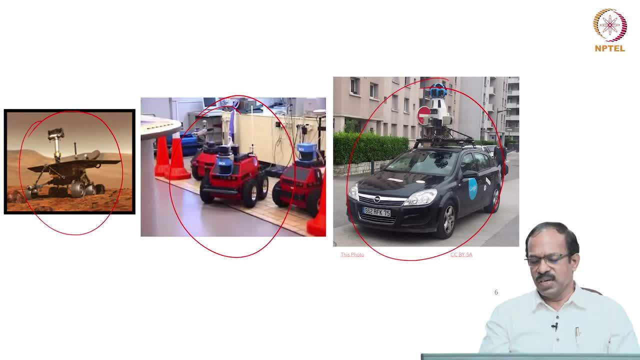 the latest trend in mobile robots, which is the autonomous car. So there are a lot of autonomous automobile companies trying to develop autonomous cars by adapting the technologies available in the robot- Yes, In the robotic field, and then using it, integrating them with the automobile system in order to 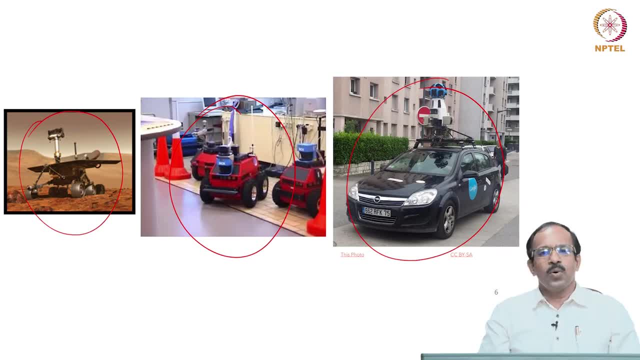 get driverless cars, So the sensing and perception is the most crucial in the case of such robots. Most of you know that when you want to go for, when you want to go for an autonomous car, you need to understand why, or you know to go for an autonomous car, you need to understand. 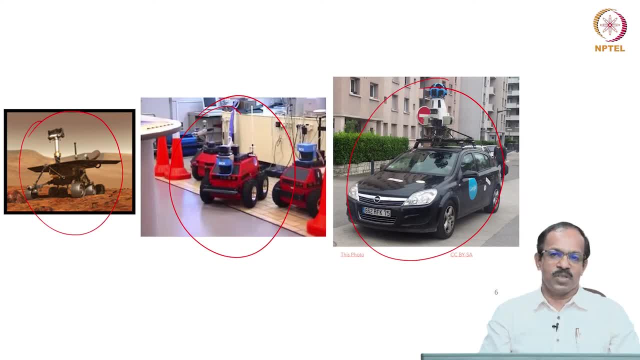 why So for a? in order to design an autonomous car, we need to know that the robot has to identify the road. the road robot has to identify the surroundings. the robot has to identify the pedestrian, has to identify the signals. 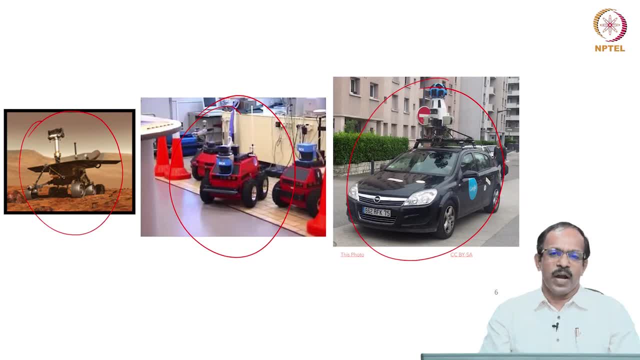 So there are a lot of things the robot has to identify from its environment, and this is possible only through sensors and perceiving the environment using the sensor data. But just before going into The sensors, let me just tell you the main difference between these two, that is, the remote. 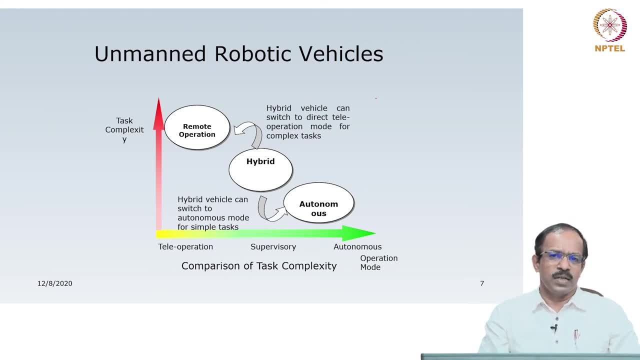 operation and the autonomous operation, and why the autonomous operation is still not coming to the level what we are expecting, As you can see from here. the autonomous robots- their autonomy is very high compared to the tele operation or the remote operated robots, but you can see the task complexity is very 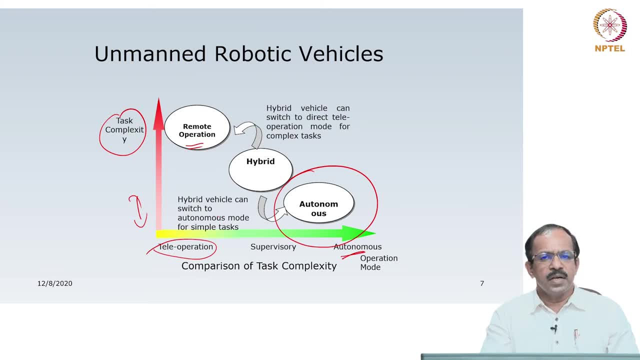 less. So it is actually very less here, and if you want to bring this to the next level, we need to provide more capabilities for the robots, And one of the challenges in developing autonomous robots, or one of the challenges in bringing the these robots to the next level, is basically: how do we actually ask, allow the robots to. 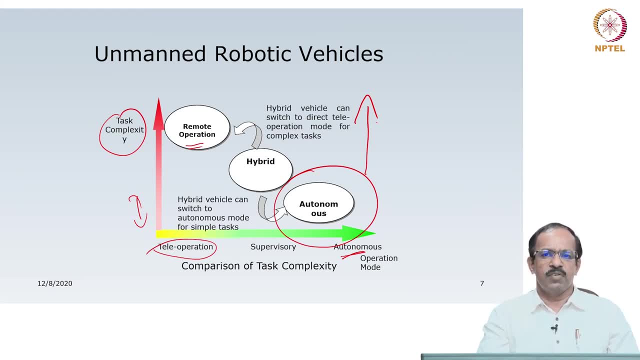 perceive its environment and take decisions the same speed as what we humans do. As a human, we actually take a lot of decisions. we actually get a lot of sensors, sensor information from our natural sensing organs, but the robot is not able to do it as fast as we can do. 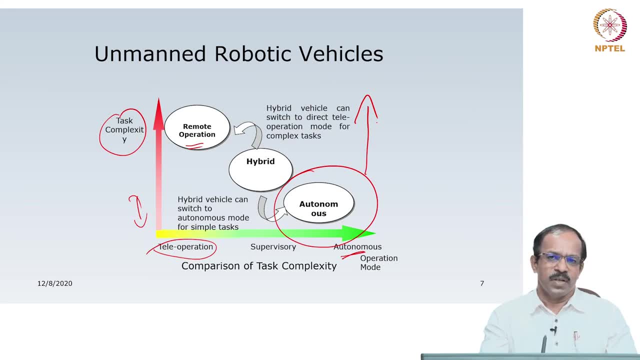 And there are many challenges in that, because the robot has got sensors which again work based on the principles that we have like whether it is a sound based or light based sensors. So the sensors are not very accurate. sensors are not able to give you the desired accuracy. 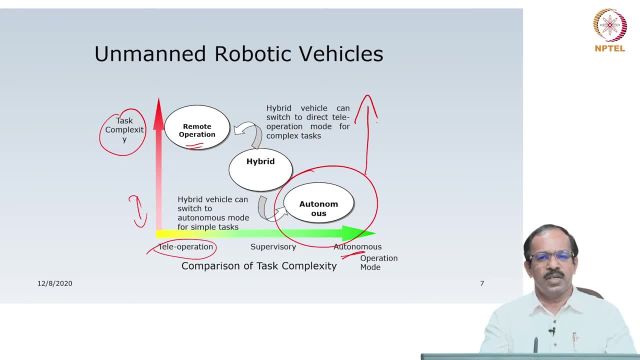 As well. the robots are not able to. the sensors are not capable of distinguishing between different objects many times. So all these are actually creating problem for autonomous robots. So one of the main challenges in developing autonomous robot is basically providing a good perception of the environment at the rate at which the human is able to perceive. 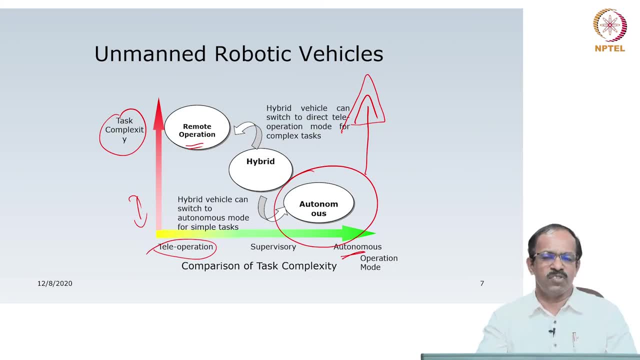 what the human can do. So once that is provided, then the robots are capable of executing it very fast. But unfortunately our sensing and perception itself suffers from many things. So we need to have better methods and better algorithms to take the autonomous robot to. 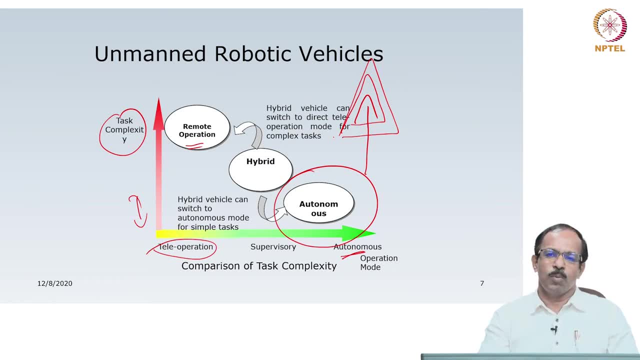 the next level of complex task complexity, where robots can work without really. I mean robots can do complex tasks without having any intervention from the human. So the telehealth is a very important aspect. It is a very important aspect. It is a very important aspect. 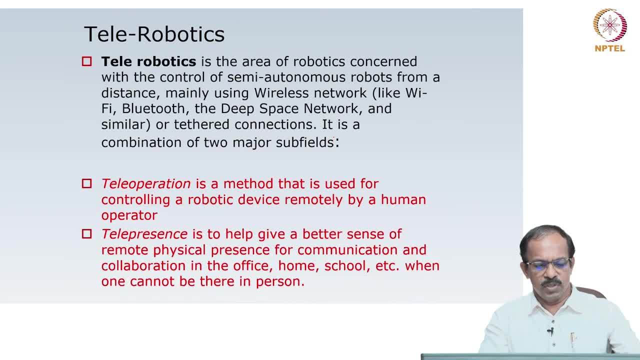 So teleoperation, as I mentioned, there are two things in teleoperation, that is, the tele, two things in telerobotics. one is known as the teleoperation, the other one is the telepresence. So teleoperation and telepresence are part of the telerobotics. 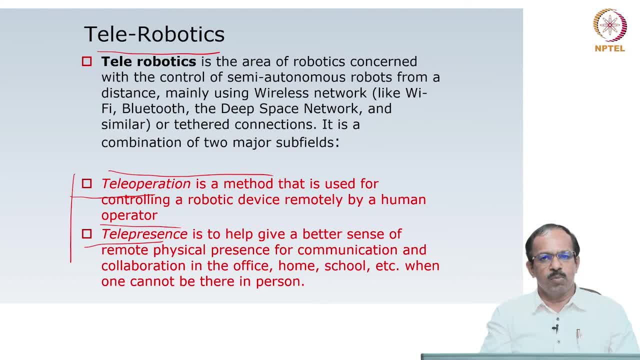 And in teleoperation we just give the command to the robot and the robot will actually execute the commands. But what we need the telepresence where the robot needs to work. So we need telepresence, So we need telepresence. 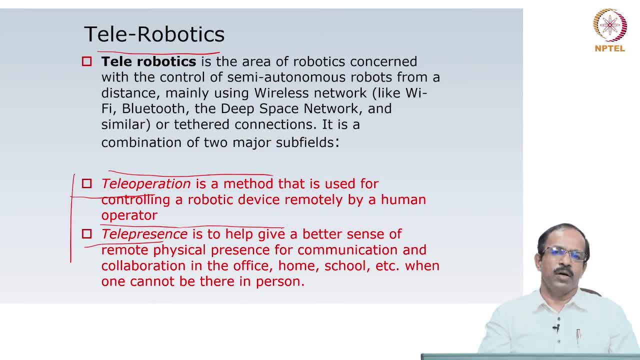 And if we want to give the give feedback to the operator about its surroundings, around this environment, we need to have feedback and this feedback comes through sensors. So here in telerobotics, the sensors basically function as data collection points or data collection devices which will just send the information back to the operator and operator. 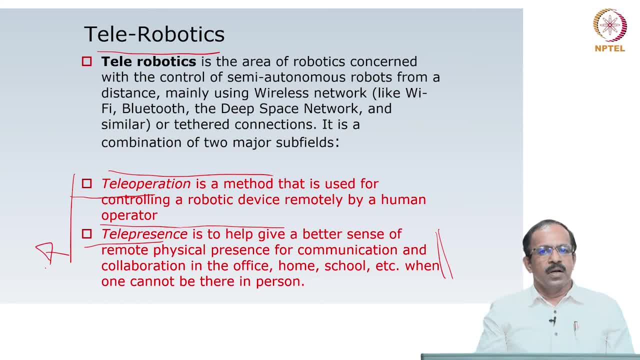 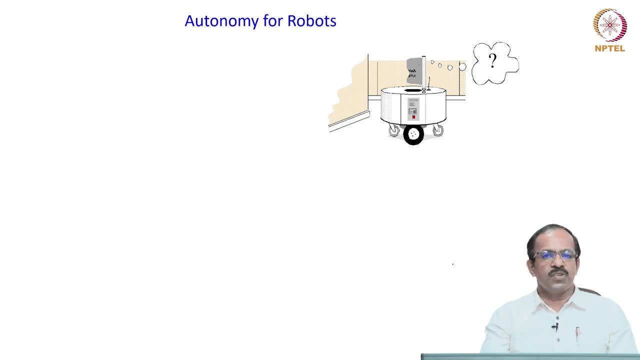 do all the processing of the data Okay. in telerobotics, the role of sensors is very limited. You need to have many sensors, but the role of sensors are very limited In the case of autonomous robots. just collecting information is not sufficient. Sensors can still do the same thing as in telerobotics. 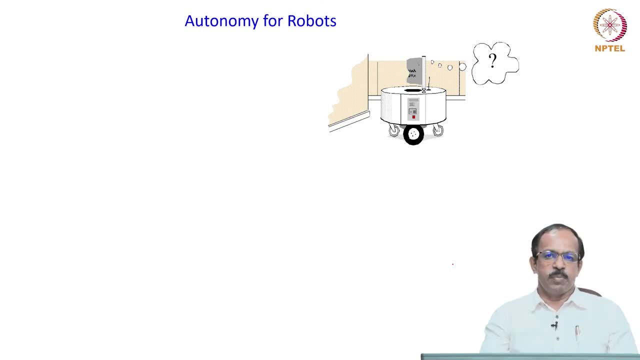 can collect the information, but processing of information is very important. So what are the things that we need in a robot? If we can understand that, then we know the importance of this. sensors play, or the sensory and perception play in mobile robots. So for autonomy for robots. so if I want to give autonomy to robots, 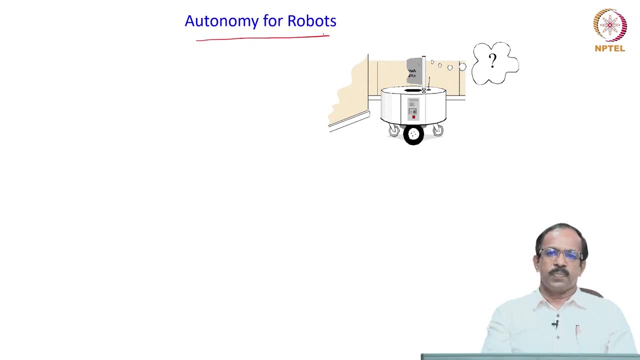 we need to understand how an autonomous system work, Assume that I mean we are all human, human beings. we are autonomous systems, So we do many things autonomously. we do not depend on any other person to take decision, So we actually get the information. 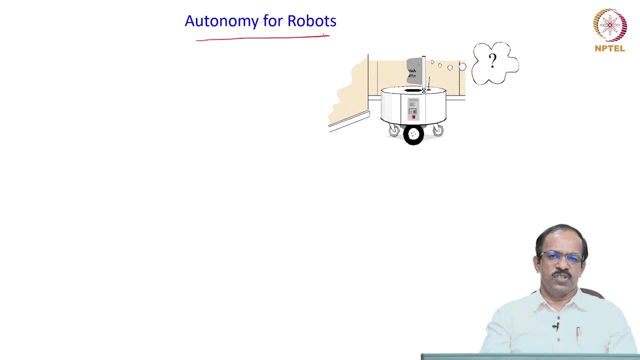 from the computer, the data, the information that is available to us, For example, if we surroundings, and then we take decision, and then we execute the decision. That is what we do normally in our day to day activities. If I had to go to some place, I will, or if I need to. 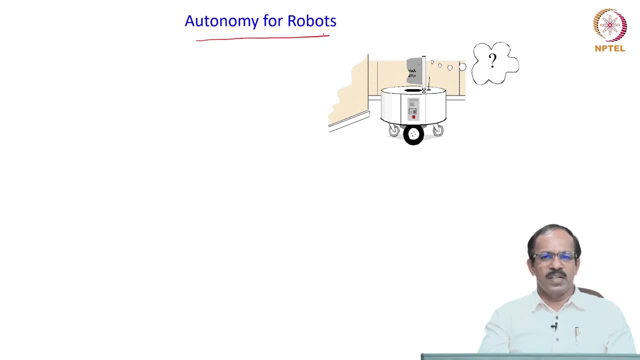 get something done. I will look at what are the things around me and then, based on all the information, I will process that information, take decision and then execute it- A robot. when you want the robot to be autonomous, we need to make sure that the robot is also able. 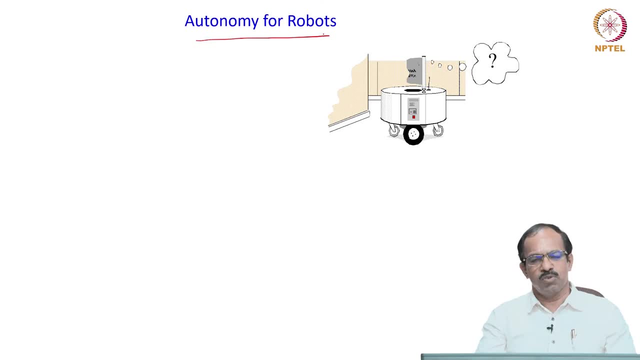 to do the same thing Because there is no human intervention, the robot has to do the task on its own. Now we need to know what are these capabilities for the robot to be autonomous. So the first thing, what the robot need to know. 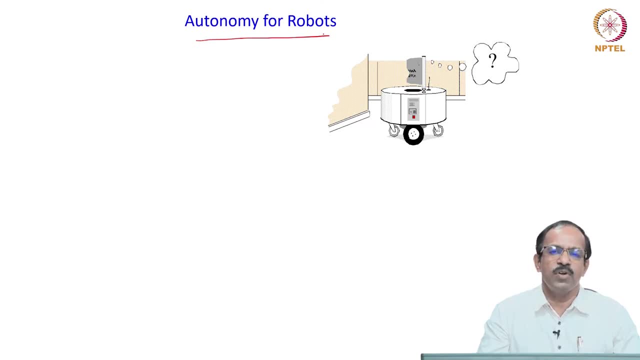 or what the robot, the capability, what the robot need to have is to see or to understand. where is it? So the robot should be able to know: where am I? So there are three, three capabilities, three key questions which a robot should be able to answer in order to be autonomous. So 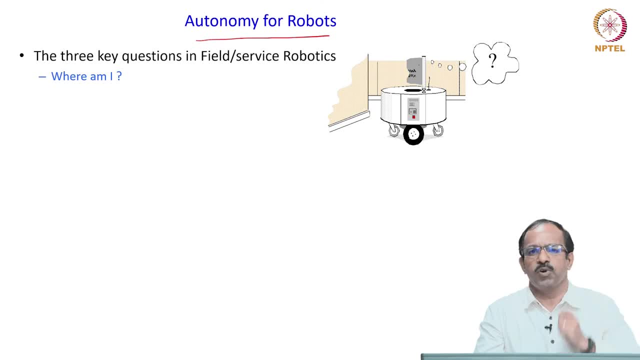 first one is: where am I? So what is the current location of the robot in an environment? Where is its position? What is its position is to be understood. That is the question: where am I? The next question is, of course, the where am I going? 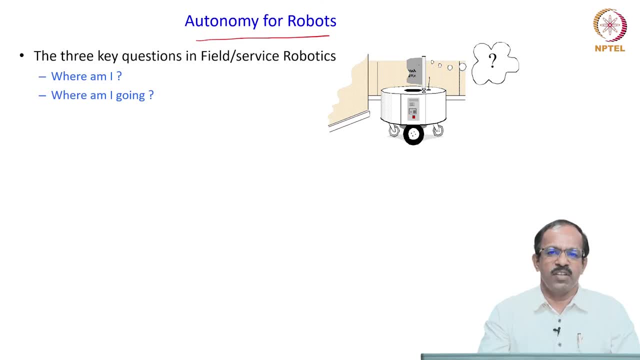 What is the target for me or what is my destination. So this actually comes from a mission planning or the robot. the user would have planned it. So once the robot knows where am I and where not, where am I going? So if these two are known, then the robot has to decide how. 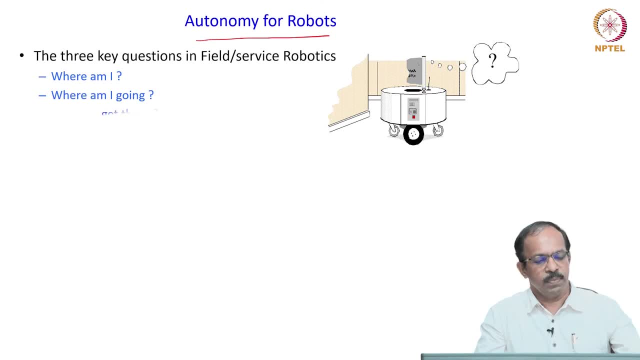 can I get there? So that is the next question. So where am I, Where am I going, How do I get there? If a robot can actually answer these three questions, then the robot is autonomous. How can we make this robot understand? 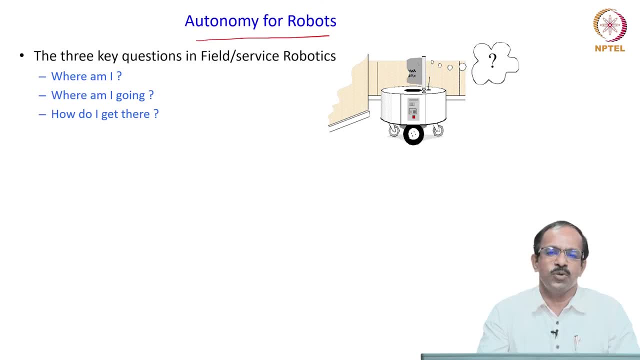 these, or answer these three questions, is the critical issue in autonomous mobile robots. For any autonomous robot, these three questions are very important And we know that we are capable of doing this, even if it is an unknown environment, By looking at the surroundings, collecting data from others or from the surroundings we will be 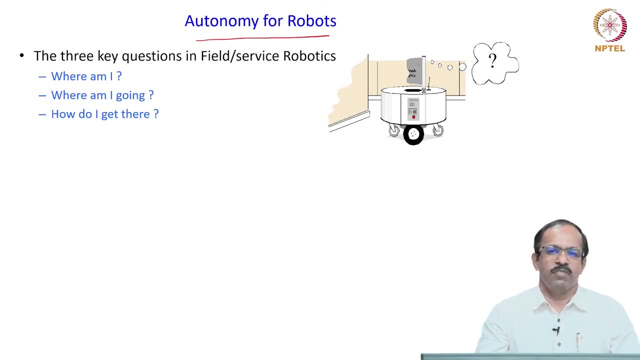 able to identify where we are When you are in a totally, when you are left in a totally unknown place and you do not know where you are. you will be able to identify where you are When you are in a totally, when you are left in a totally unknown place and you do not know where you are. 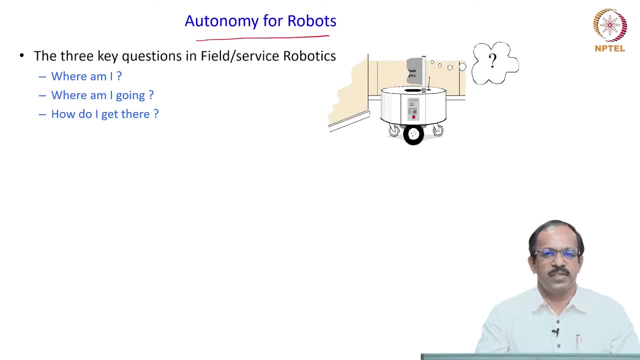 you will be able to identify where you are. Then what you will do? you will just go around and then try to look at surroundings, look at for signposts or some landmarks And based on all this information, you will decide. you will make the decision that you are. 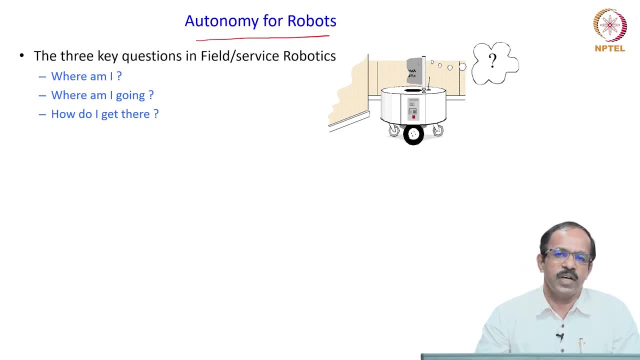 in the correct particular location. The same way, robot also has to do it, And for that the robot needs to have sensors. the robot needs to capable of needs to be capable of analyzing the sensor signals and then taking decision based on this data. So that is what actually needed. So 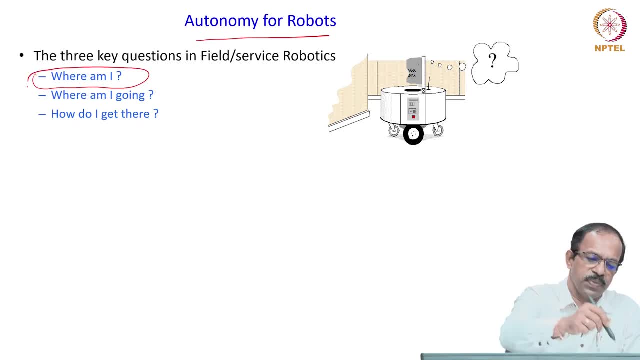 the first part. this part is very crucial for a robot: where am I? And that actually can be given only by sensors and the sensor data. So that is where the first thing comes into play, And how do I get? there actually is a question of path planning and execution of path through. 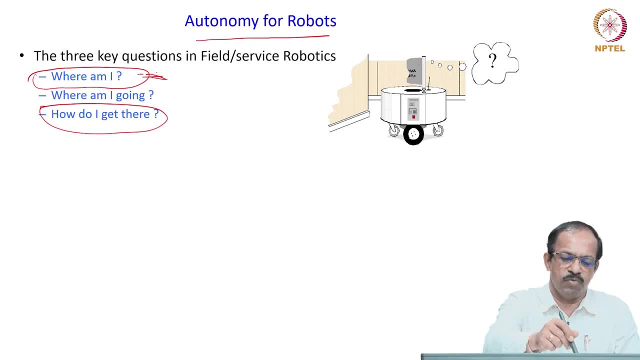 controlled signals and other things, But the first part, the answer of where am I, is to be answered, And this one, many times we call it as the localization of a robot. So to answer this question, the robot need to have a model of the environment. 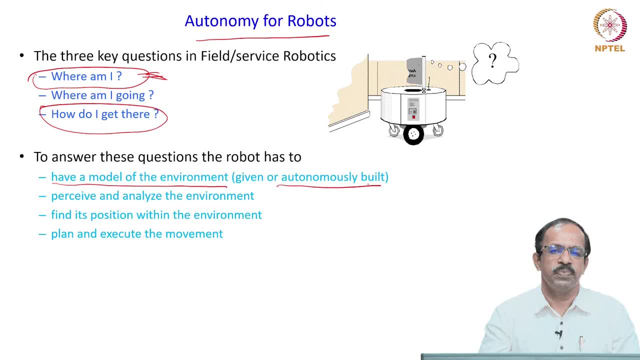 given or autonomously built. So the robot needs to have a map of the environment. a digital map is given, or the robot should be capable of building a digital map. So that is one requirement for the robot And then, within that environment, it has to perceive and analyze the 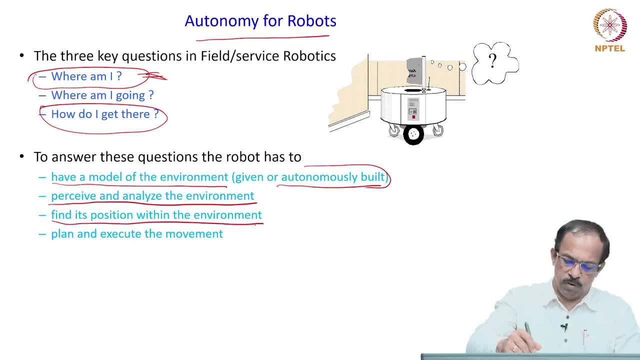 environment and then find its position within the environment. So this is basically known as the localization of a robot. the robot needs to localize itself. This is the requirement of a robot when answering the question. where am I So if there is a map? 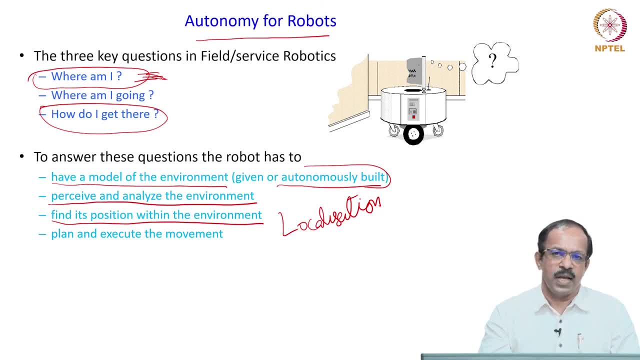 then use the map and the information coming from the sensors, analyze this and then decide where it is is the first thing, And then plan and execute the environment. It has to plan and execute the environment, And this one, basically we call this as the localization of a robot, It Σ. 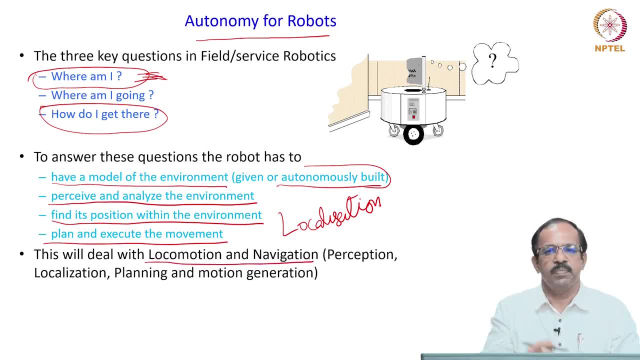 be defined as here. If you press this button, the system will go out. then it will look up for the this as the locomotion and navigation of the robot. So for any mobile robot we need to have a locomotion and navigation mechanism. 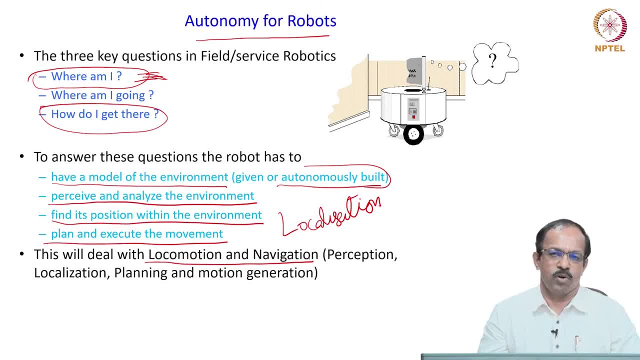 This is to be built into the robot in order to make it autonomous, And that is the job of the designer: to ensure that the robot is capable of doing this- locomotion and navigation in an environment. then only we can make it autonomous robot, And this can be achieved through these 4 steps. that is the perception, localization, planning. 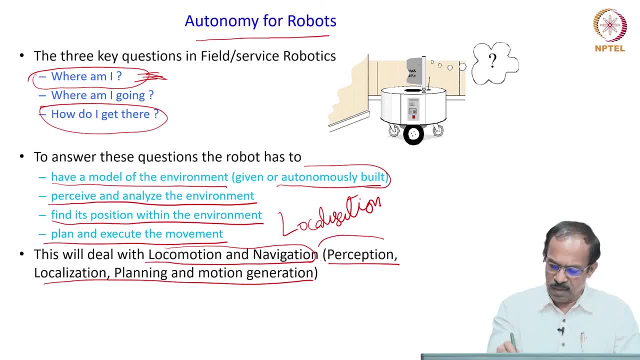 and motion generation. So perception is the one which actually help the robot to collect information from the surroundings using sensors and then perceive its environment, analyze its environment and then localize itself. So it uses sensors and then sensor data, analyze it and then localize it. 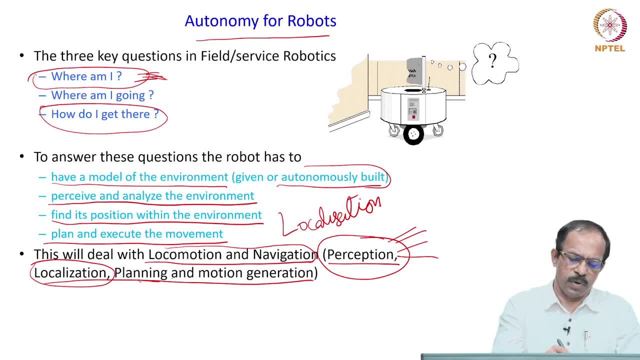 And then try to localize itself And then, of course, the planning and motion generation. So these are the other steps that the robot has to do. So it basically- I am just explaining this basically- to tell you that any robots need to have this capability of perception and localization in order to have autonomous capabilities. 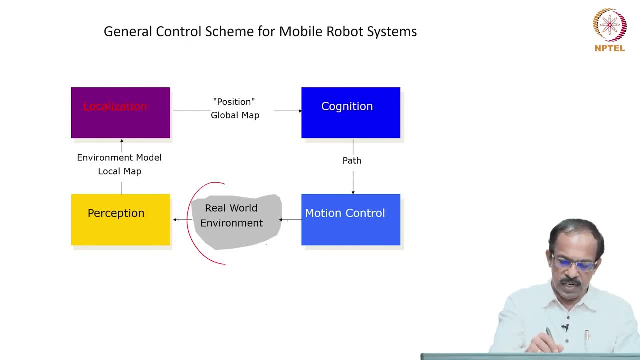 So this has been explained here. So if the robot is in the real world environment, the perception process will help the robot to analyze the environment and then it should be able to do the localization And then, based on the current position of the robot and where it has to go, it has to. 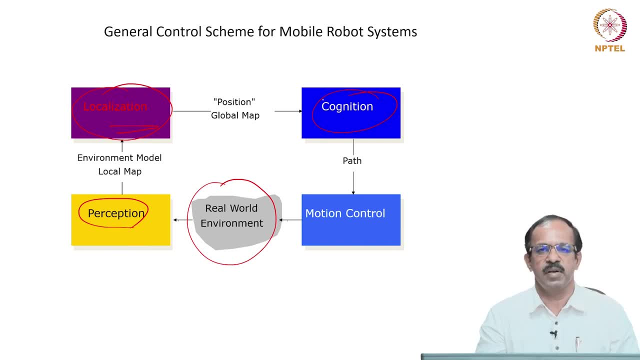 process. this information cognition is the processing of information and taking decisions, and that will generate some path and then, based on the path, the robot will be having its motion control and it will start moving in the real world environment. So this is the way how a mobile robot will be moving in its environment. 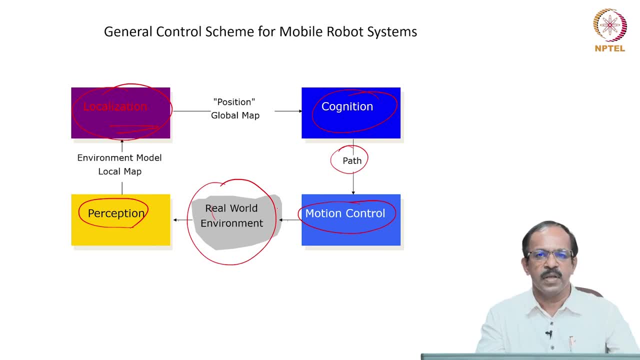 And this will be a continuous activity. It will continue, it will be working on a cycle. So this is the way how a mobile robot will be moving in its environment. So this is the way how a robot will be moving in its environment. 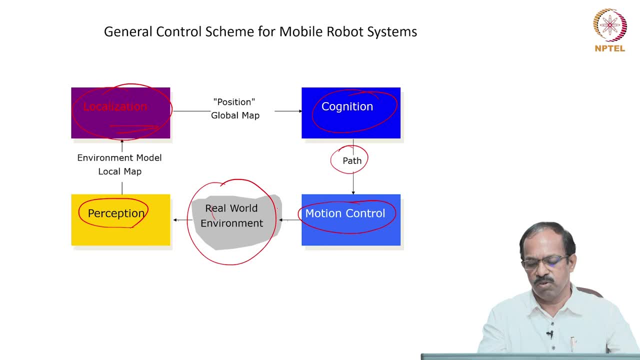 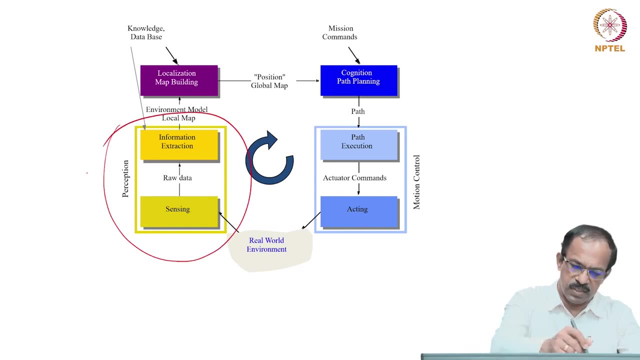 So this is the way how a robot will be moving in its environment. So this is the way how a robot will be moving in its environment. So every step, this will be continuing the perception, localization, cognition and motion control. So let us look at this perception part, because that is of interest to us. 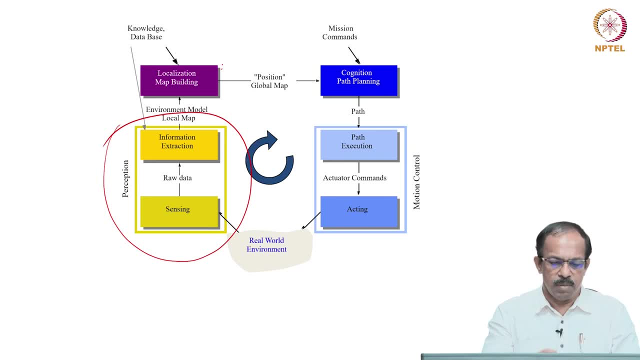 We will talk about localization slightly later, but perception is the first part. So perception includes the sensing and information extraction. So sensor will be giving you the raw data and from the raw data you need to extract the information. So how do you extract? the information is important and what are the challenges in extracting? 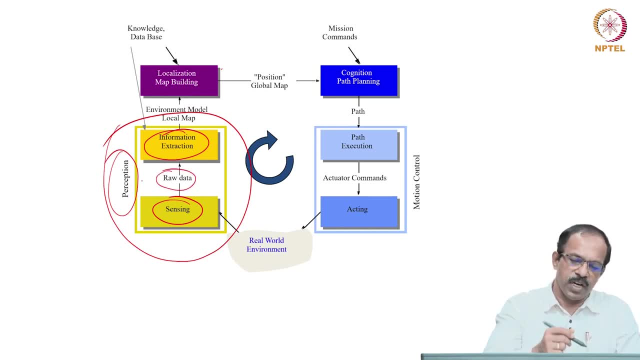 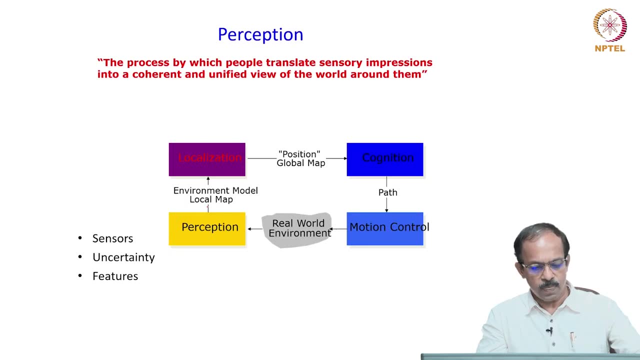 information is important, But even getting the raw data. there are many challenges in getting the raw data So we will look at those issues as we progress. So the sensing part, the perception part, we can see that the sensors are the main element. 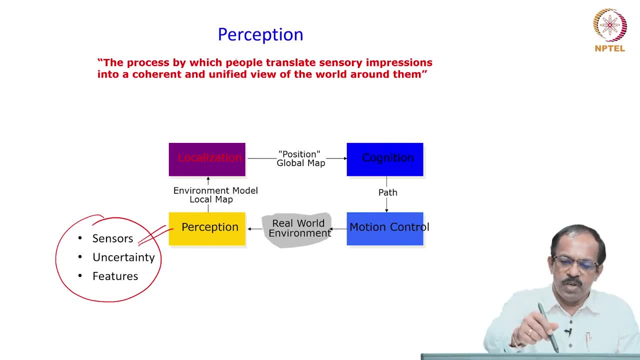 in the perception. Okay, So the process by which the people translate sensory data, So the process by which the people translate sensory data, So the process by which the people translate sensory- infant, персонal and sensory 설�atic classics- into concurrent and unified view of the world around them is known as perception. 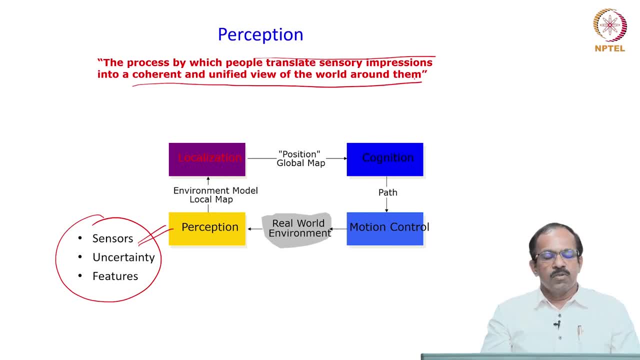 So this is what actually the robot need to have the perception capability. So how do we process the sensory impressions? We have many sensors, or the robot has got many sensors, So how do we actually process these information, the sensory impressions, and then how to convert? 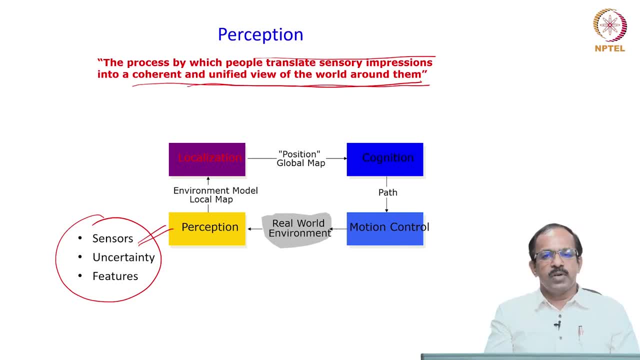 that into a unified view of the world. So you need to create a unified view of the world, or the environment, environment, and that process is known as the perception process. So there are two things: one is the sensory impressions, the other one is the conversion. 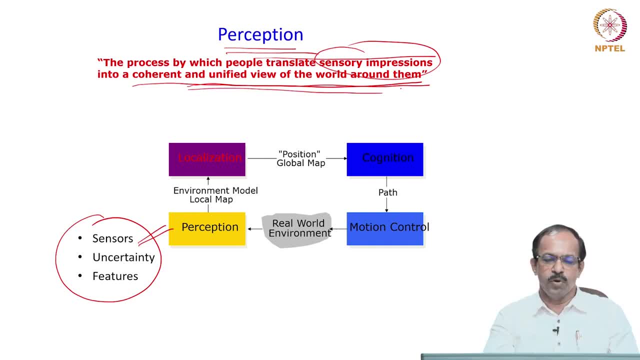 of that into a coherent view or unified view of the environment, and that is done through sensors. So sensors are the first element which actually collect the information, so get the sensory impression, and we use many different types of sensors to do that. But when we use the sensor, there are many challenges in using the sensors. one is about 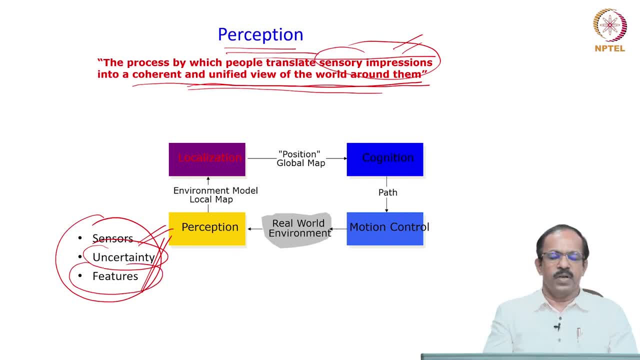 the uncertainty in the sensors and then the feature extraction, of feature extraction from the sensory signals. As human, we can actually extract many features. just by looking at once, just by having a glance, we will be able to extract many things in the environment. for a robot it is not. 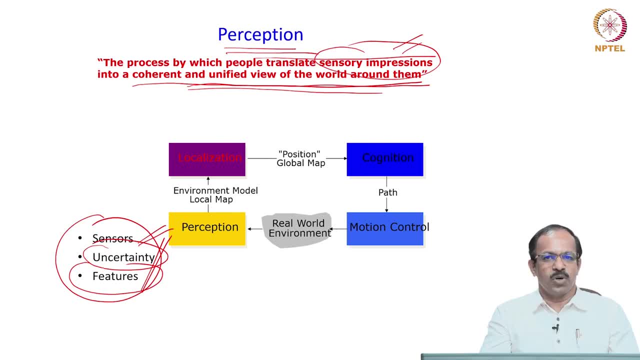 possible because its sensor does not have any intelligence on its own. It will just give you a raw data. it is up to us to interpret what is actually there on the on the scene. and again, this information changes depending on the lighting condition, the temperature, humidity and many other conditions. 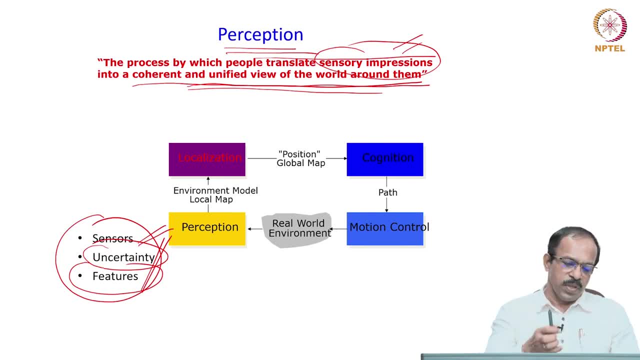 And the robot is not able to distinguish between these variations also. So, unlike a human being, who can actually distinguish many things, even in a sunny day or in a cloudy day, Or during rain or during mist, we will be able still be able to distinguish things. 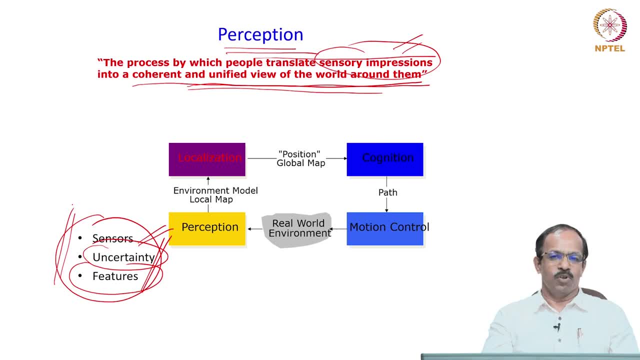 when what we are seeing, That may not be the case with robots, especially because of the sensor limitations. So that is what actually we need to understand how the robot can actually do this, even under different conditions, or what can be done in order to have the robot the capability to. 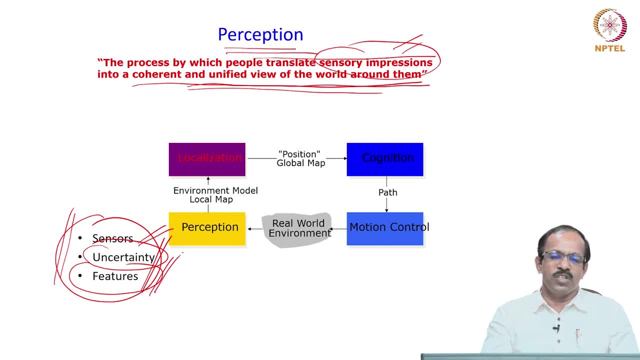 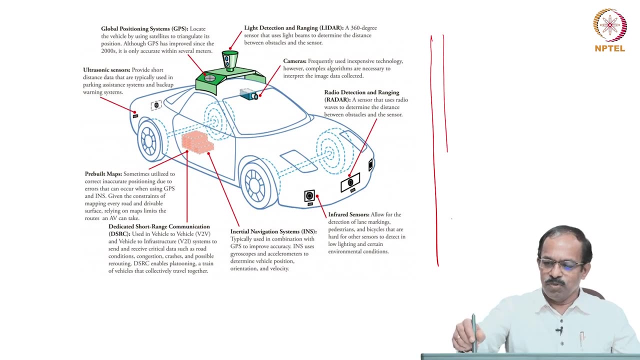 overcome these issues and still do a decent job of perception and give a good feel of the environment. So that is what actually we need to understand. So you can see, in order to do that- suppose you want to give a perception of the environment- 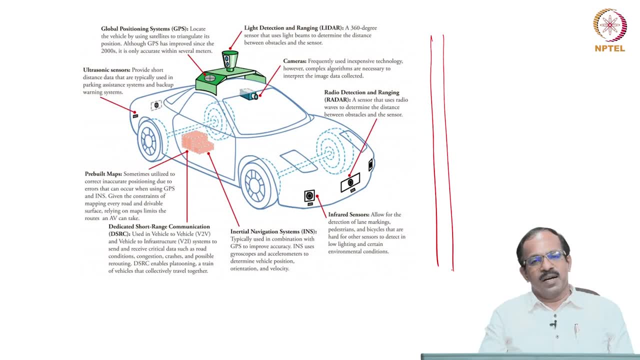 to the robot. in the case of a car like this, an autonomous car, you can see there can be so many. there need to be so many sensors, So something for the positioning system. so you use a GPS sensor, then for ultrasonic. 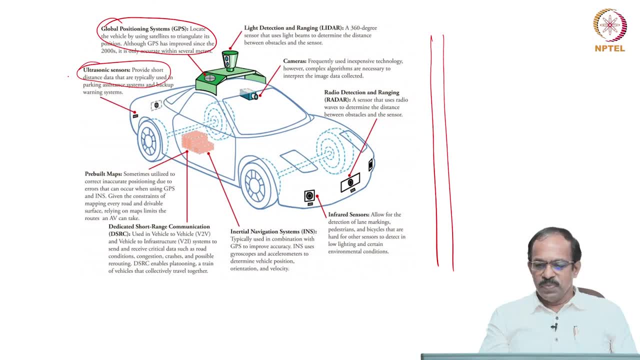 sensors to look for obstacles or objects around, Then you have the radar, and then you have the cameras. you have the SLDR and the infrared sensors, air chill navigation system and dedicated short range communication and many other things also. See you, can you need to have so many sensors in a in a robot in order to get the information? 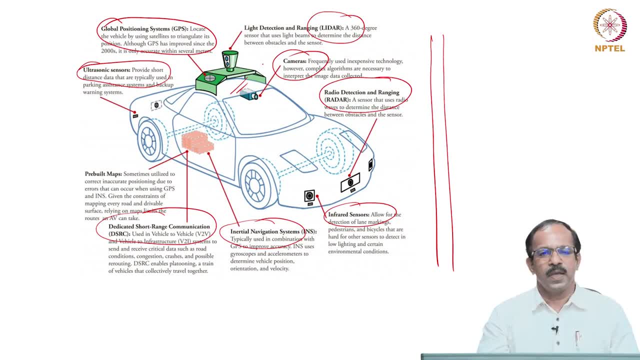 from the surroundings. Now, when you have so much information, we need to process all this information in order to get the, get the perception of the environment. And when we have to process all this data, then we have to little bit of dude here here. 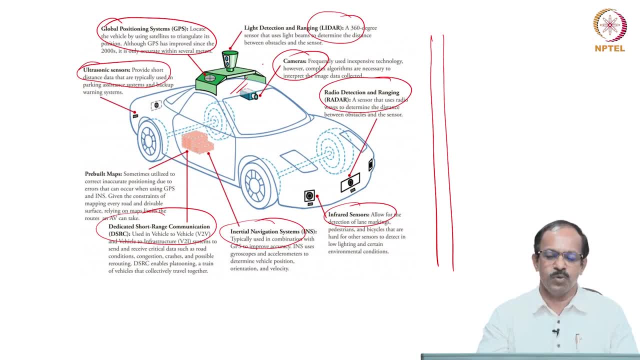 What was you guys talking about last time? About the назывation, this information. it takes time also, And that is why many robots are very slow. many autonomous robots are very slow because of the large processing of information and then trying to overcome the uncertainties and then have a good estimate of the surroundings. that takes a long. 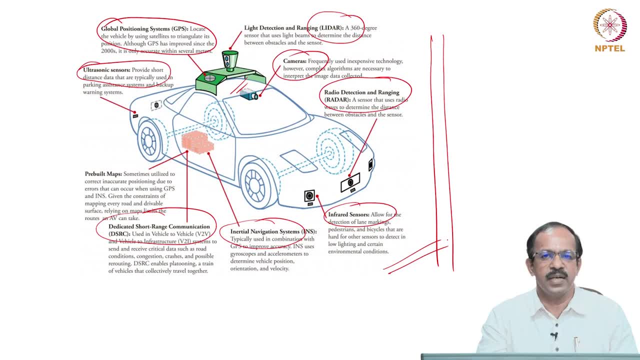 time. So that is one of the reasons we have still have difficulty in having a fully autonomous system or fully autonomous cars on the roads. This: there is a talk about autonomous car, or there are a lot of people talking big about autonomous cars and you must have heard about 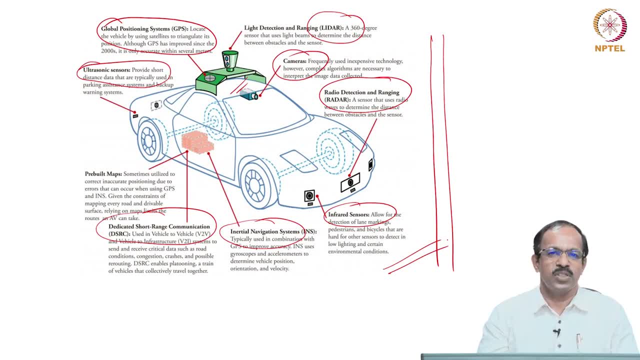 Google car, which is already undergoing trials on the roads, But it looks like we are still far away from having a fully autonomous car which are which can be commercially operated on the roads. Maybe it will take 10 to 20 years before us to get. 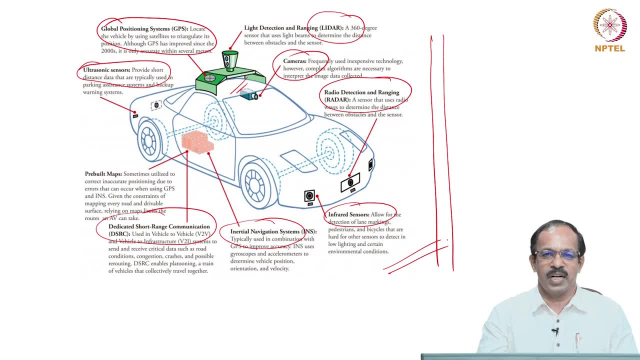 a really fully autonomous, driverless car on the roads because of the challenges involved in many things and many uncertainties are there And the environment is highly unstructured and robots are not capable of handling the unstructured conditions. So once you have a very structured condition, the robots are very good to do work, but the moment it goes unstructured, then 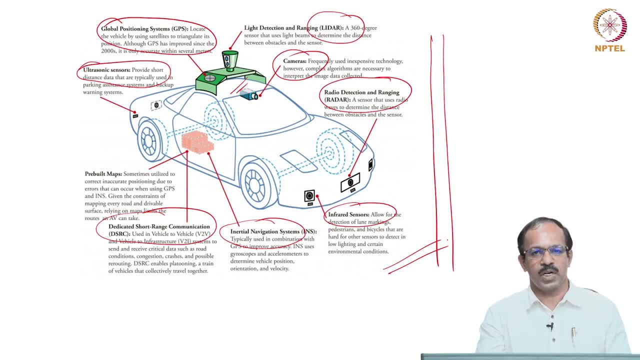 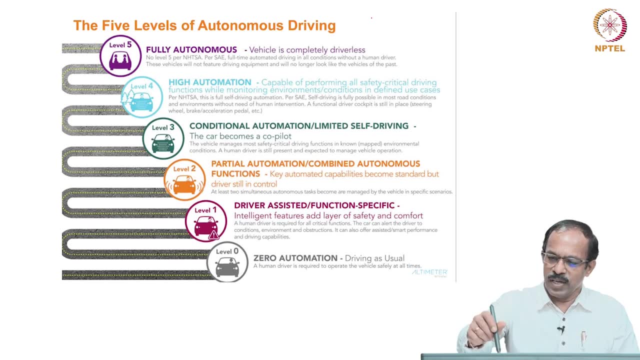 things become very difficult. So these challenges need to be overcome in order to get a fully autonomous robot. So the full autonomy is, as I told you, it is far away, but now we need to go by, step by step. So driver assisted functions are one way to move forward. So you might have heard about these. 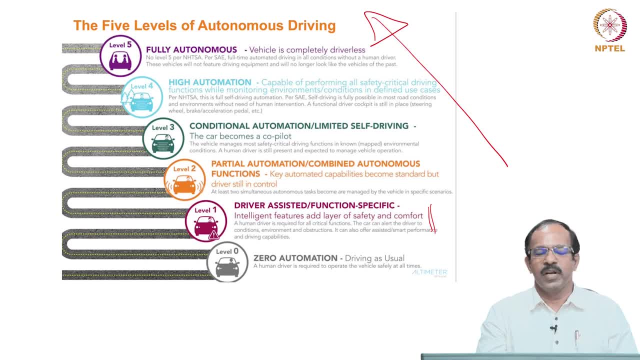 cruise control and other features in cars where actually you can fix a speed and then the car will be going at that speed, Of course without much of an intelligence, but then we can actually add intelligence. the car can actually identify the. there are cars which can actually identify the. 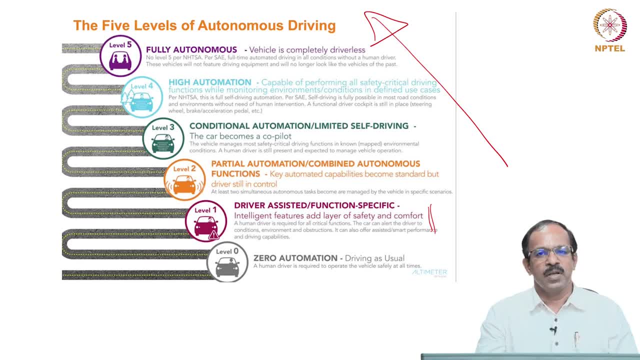 curves and then go in the middle of the road. So like that we can add a little bit of intelligence, that is basically the driver assisted functions, And then as we go up, we will be adding more and more autonomy to the robot and finally we will become a. 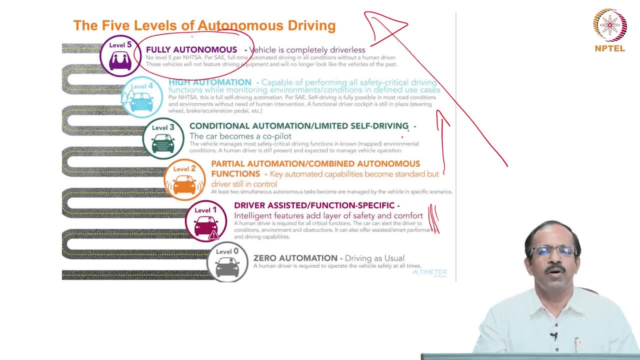 we will have a level 5 autonomy, or we call it as the fully autonomous car. So it is a long way to move forward, but we are already in the level 2 this stage. but I think we will be moving forward and get into the level 5, maybe in 10 or 15 years. 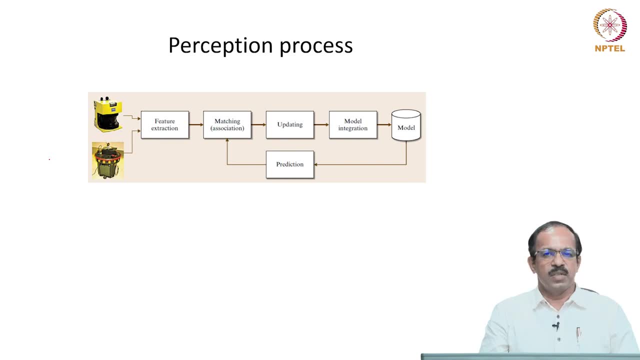 So that is about the general introduction, about the importance of having sensors and perception and why we need to have a good perception systems in the mobile robots. So before going to the sensors, let me just tell you what is the perception process itself is. Anyway. 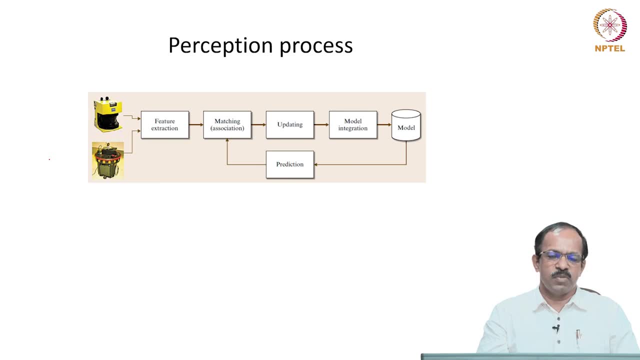 through these steps in detail. but the perception process basically involves the sensors. So we have the sensors and then sensors will take the information from the surroundings and then give it to the robot. Then the robot controller will just extract these features from the data. Suppose the camera sees an object. it will try to identify whether it is a tree or 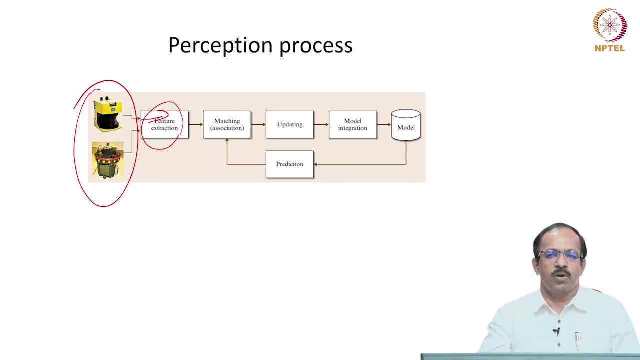 it is a wall, or it is a human or a car or whatever it is. Similarly, these radars also can identify many things, like the walls and other objects also. Now, this will be a raw data coming from the sensors and then that this is to be processed. 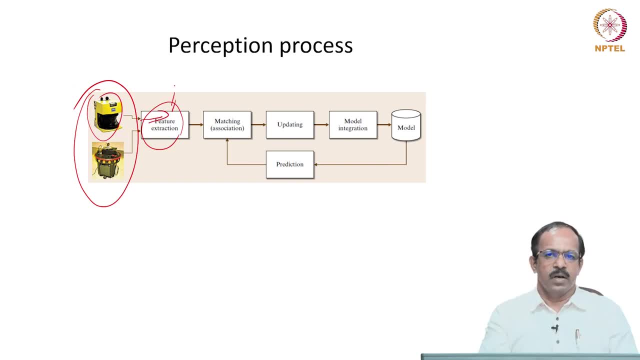 and we will extract the features and identify: there is a wall at 5 meters away from this location or at a particular orientation. That kind of information can be generated. that is basically known as feature extraction. Now, with the feature extraction, we get a feature and then it check whether it is actually. 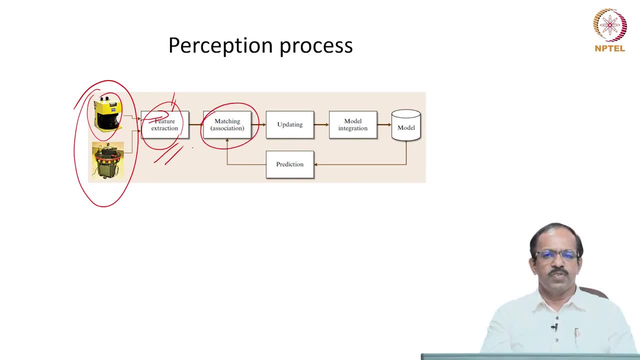 matching with something already given to the robot. So if the robot is given a map, it will check whether there is already there or it is a new feature that is coming and that will associate itself, And if it is not there then it will update the database. it is on a map given. 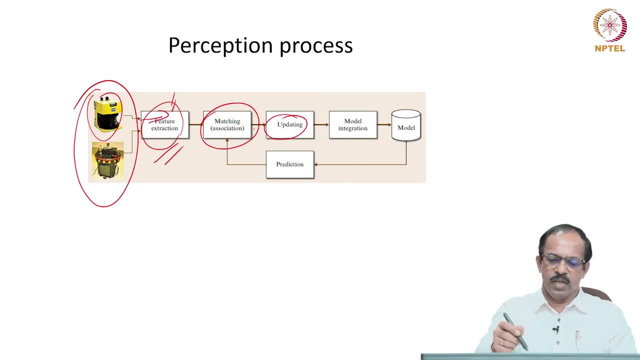 to the robot. It will update, create a map with the updated information and then it will integrate with the environment model or the model of the surroundings And then, using the map itself, it will say: now the robot is moving. then the robot will. 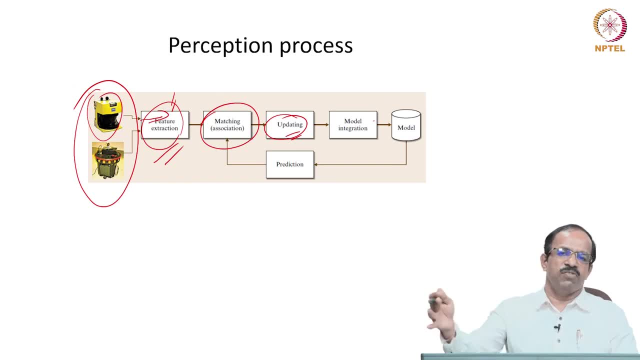 because there is a map already. so it will predict something you can see after some time, And then that is basically the prediction. the robot will be able to predict that now, if you are in this location, you will be able to see something based on the model that is available. 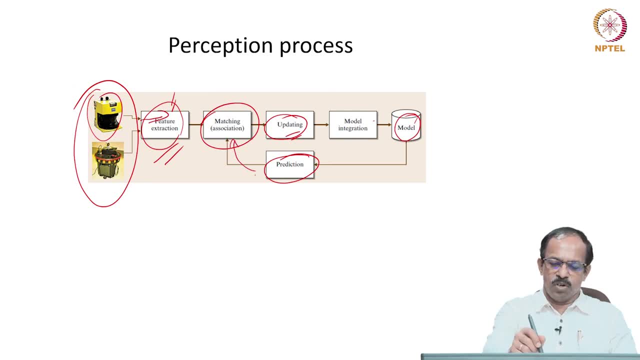 And when the robot is seeing that one, it will actually check whether it is seeing it or not, And if it is seen, then the robot is in that position. If it is not, in some it is not able to see, then something is wrong with the position estimate, or it is. 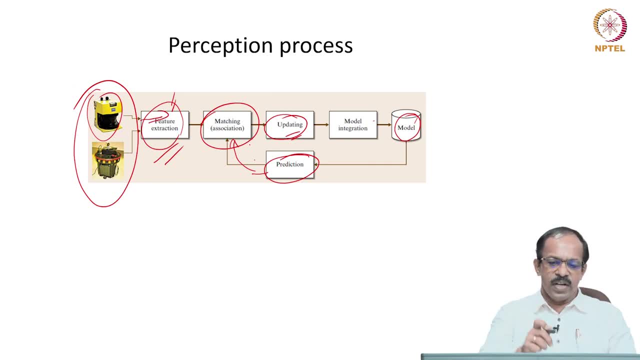 the surroundings of the robot has changed And this process will keep on happening. it will continue throughout the operation of the robot and continuously the robot will be looking for information using the sensors, extracting the features matching with the model and then updating the model and then keep on predicting and 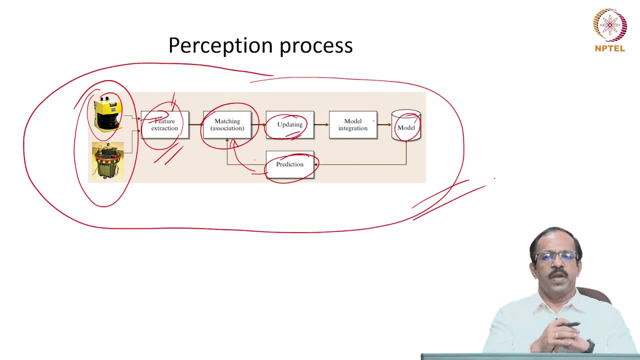 updating it. So this process will keep on happening in the robot in order for the robot to get a good perception of the surroundings And that actually that perception allows the robot to do its localization and all other activities. So the primary thing for a robot need to have is 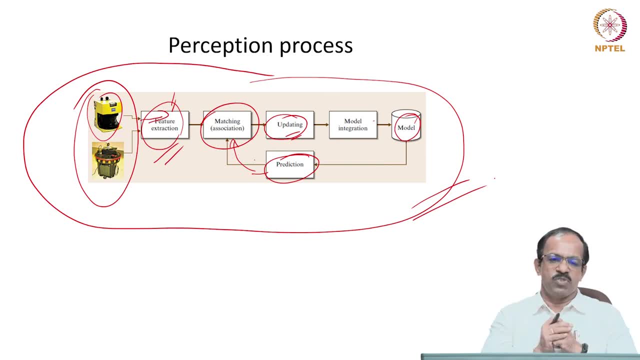 the perception- a perception of the environment- And that perception comes through sensors and then processing of this information and following the perception process. So this is what we are going to learn in the next few lectures: How the sensors can be used to collect the information and how this information can be processed to get the features. 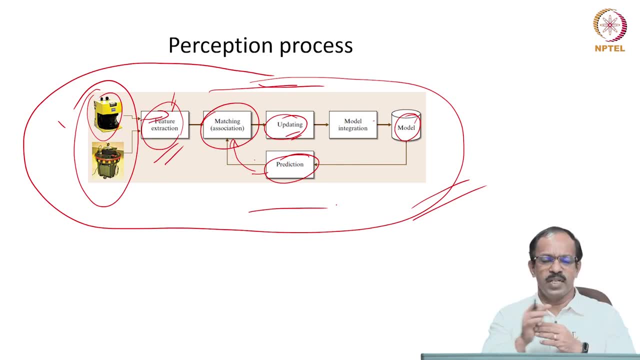 Of course there are many feature extraction exercises which we will not be going to in detail. just want to explain few things And then we will see how the information can be used for localization of a robot also. will stop here for this session and continue this in the next lecture. Thank you.